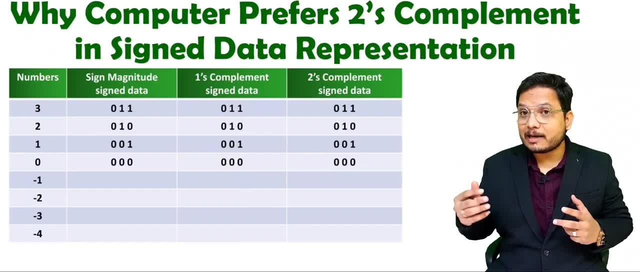 one's complement signed data representation method. And third is two's complement signed data representation method. So, out of these three, why should we have two's complement method? So for that, let me explain you first how normal signed data representation method is there. 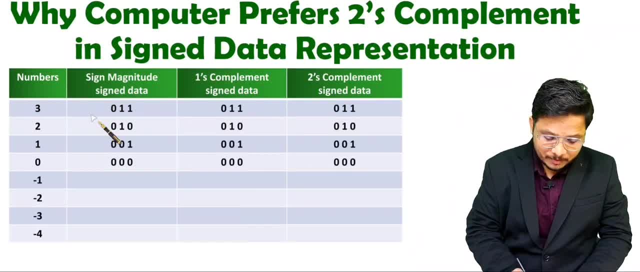 So if you observe here in normal signed data representation method, we are having positive numbers over here And then we are having negative numbers over here, And I'll be considering one example in which we'll be representing data by three bits, right? So if you observe, with all 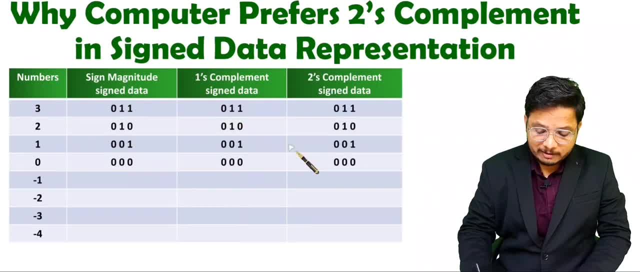 these three methods. we are having same methodology for positive number representation. right, There is no difference in representation When it comes to positive. like you see, initial digit: that is zero for all three methods. that indicates these numbers are positive And based on value only it is represented here. 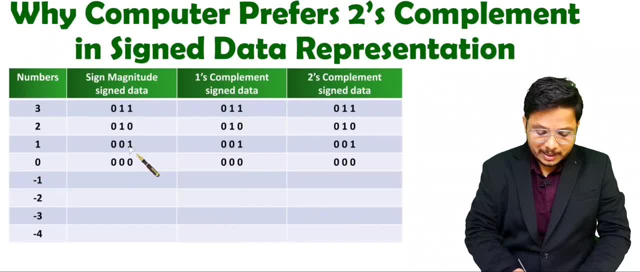 like you see, 0 0, 0, that is zero in number. 0 0, 1.. That is 1 0, 1 0 that is 2 and 0 1, 1, that is 3.. But when it comes to negative data representation, at that time you will have: 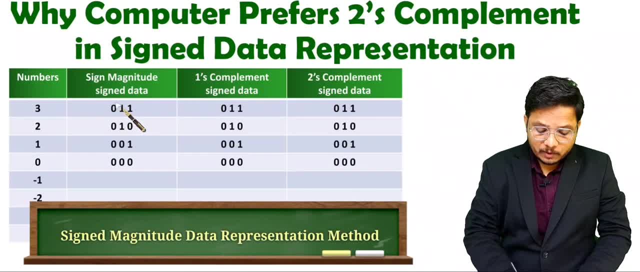 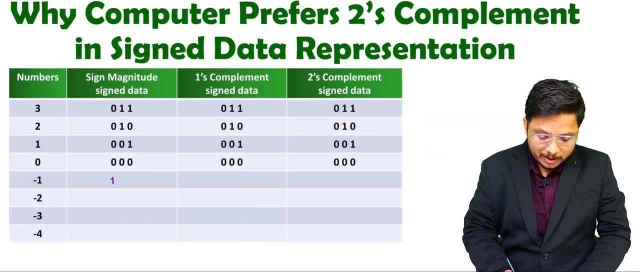 to understand how these methods are there. So for signed magnitude, signed data representation method, you will be having first digit, that will be one for negative data, right, and then magnitude will be as per last two digits right in three bits method. so see this first bit that is indicating one means it is minus, then zero one, that is magnitude right. 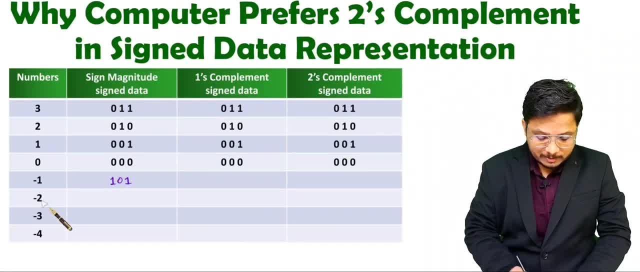 so one zero, one that you need to have it for minus one. similarly for minus two, first digit that will be indicating sign. so that is one over here for negative data and two means one zero. that is a means one, one zero. that is therefore minus two in sign magnitude. data representation method. 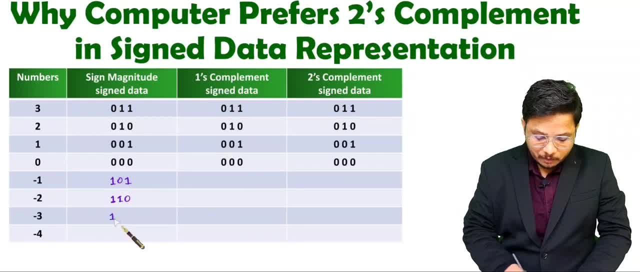 and for minus three, you will be having one. four minus and three means one, one right. so that is how normally we represent data in sign, magnitude, sign data representation and here minus four. that is not possible why the reason is four is having a. the reason is four is having a. 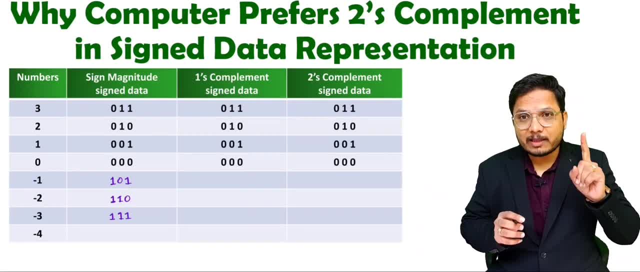 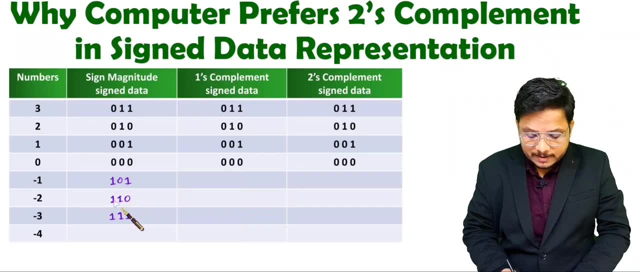 requirement of three bits, right? you see, minus is having one and then four is having one zero. zero means in total four bits are required. so here we are talking about three bits, right? so four minus four. that is not possible by three bits over here, right? so I am just marking that by cross over here. but if you observe here how many combinations that we have utilized in three bits, if you observe we have utilized seven combination, right, so which combination that we have not utilized yet over here? 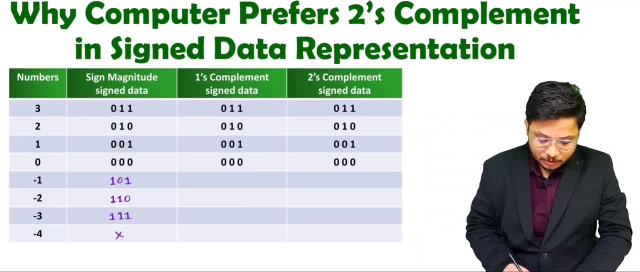 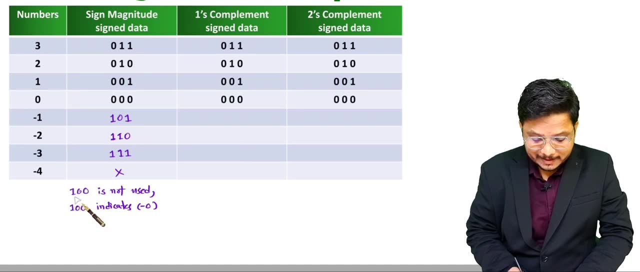 so if you observe one zero zero that we have not used, why we have not used one zero zero? the reason is: one zero zero that indicates minus zero. you see this one that is representing minus sign, and zero zero, that is a magnitude, means minus zero. so here, my dear students, what we are doing, we are wasting one digit. one zero zero indicates minus zero. minus zero is not required in number system representation. so here, my dear students, what we are doing, we are wasting one digit. one zero zero indicates minus zero. minus zero is not required in number system representation. so here, my dear students, what we are doing, we are wasting one digit. one zero zero indicates minus zero. minus zero is not required in number system representation. so here, my dear students, what we are doing, we are wasting one digit. one zero zero indicates minus zero. minus zero is not required in number system representation. so here, my dear students, what we are doing, we are wasting one digit. one zero zero indicates minus zero. minus zero is not required in number system representation. so here, my dear students, what we are doing, we are wasting one digit. one zero zero indicates minus zero. minus zero is not required in number. 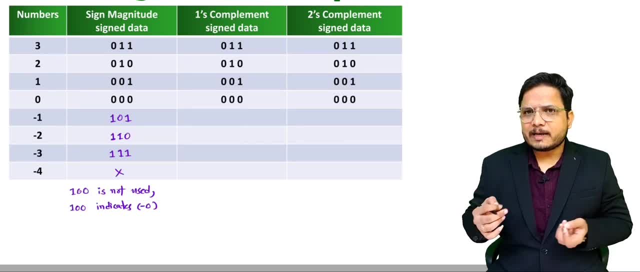 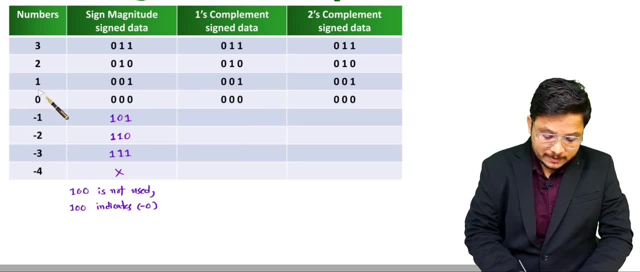 So 1's complement of this 1, that is minus 1,. so 1's complement means what: Instead of 0 you will have to place 1, and instead of 1 you will have to place 0. So to have minus 1, 1's complement of this, that is 1 1, 0, right. 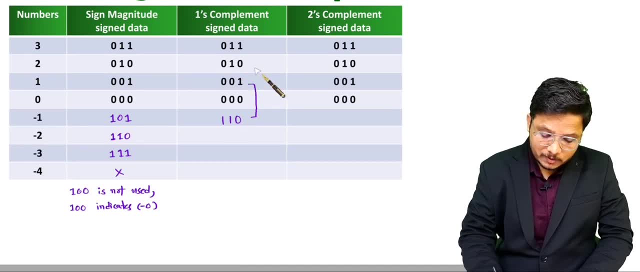 Now to have minus 2, 1's complement of 2 that you need to have, so 1's complement of this, that is, 1, 0, 1 and minus 3 that will be as per 1's complement of this. 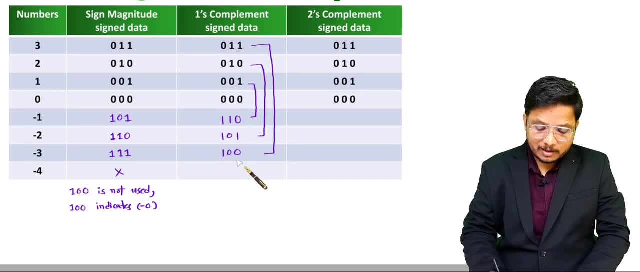 So in that you will be observing that is 1 0, 0, right. So that is how we represent data in signed representation with 1's complement method, right? So whatever data that is there in positive, in that, you will have to provide 1's complement. 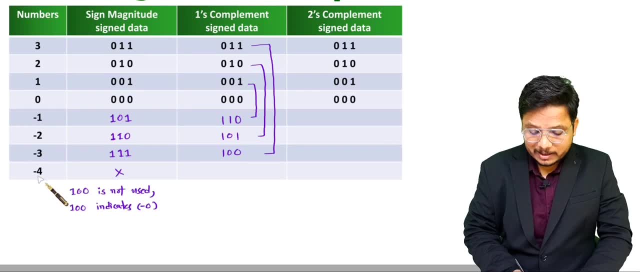 So here, if you observe minus 4, that is not possible. Why? The reason is, when it comes to minus 4, at that time you will have to take 1's complement of plus 4.. Now in signed representation, first digit, that indicates what. 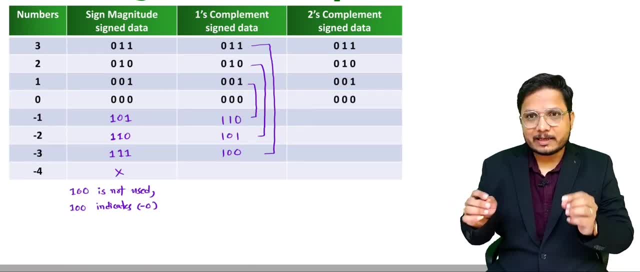 Polarity: If it is 0, then it is positive, if it is 1, then it is negative, right? So here to represent 4 in signed representation with 1's complement, you need to have 4 bits. First is 0, then 1, 0- 0.. 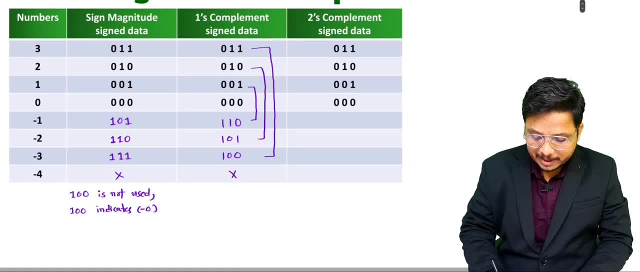 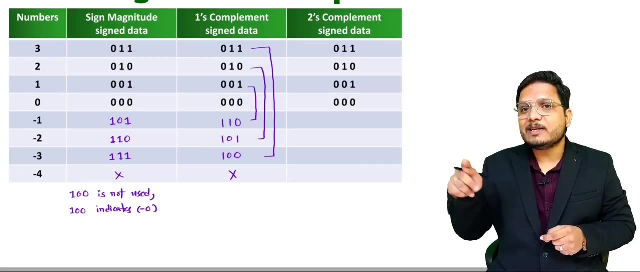 So minus 4. that is not available over here. So what I am doing is I am marking it as cross. Why the reason is: plus 4, that will be 0, that indicates positive data, then 1: 0, 0. So it requires 4 bit. 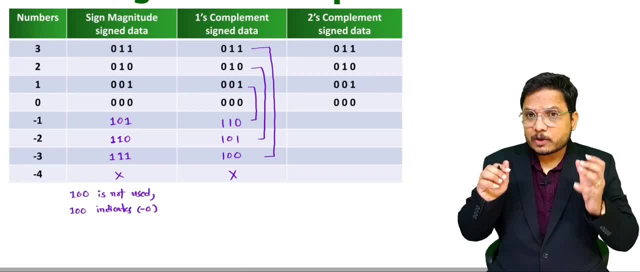 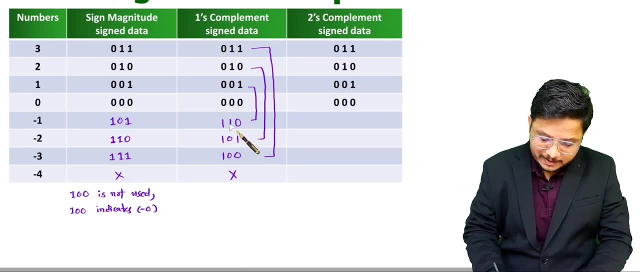 Here we are having 3 bit representation, right. So here we need to see how many combinations that we have utilised over here. So if you observe 1, 2, 3, 4, 5, 6, 7, 7 combinations that we have utilised over here, 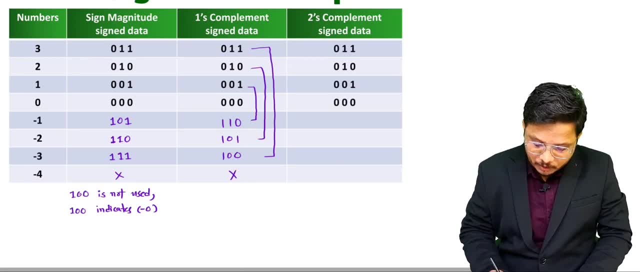 So which combination that we have not utilised over here? So if you observe 1 1, 1 is not utilised over here. You see 1 1, 1 is not utilised. Now what is the meaning of 1 1, 1, 1 1, 1, that is 1's complement of 0 0, 0 means you can. 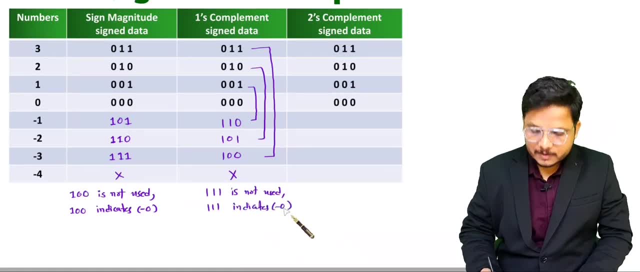 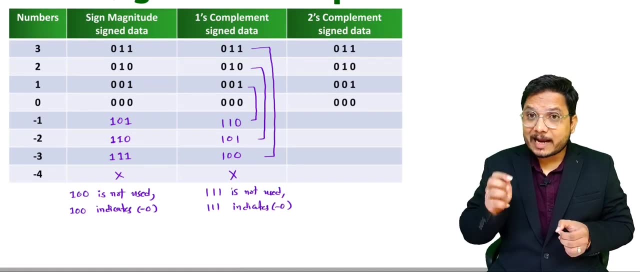 say 1, 1, 1 indicates minus 4. Indicates minus 0. So here, my dear students, again we are wasting 1 digit to represent minus 0, as it is not required, right? So in signed magnitude, as well as in 1's complement, we will be always wasting 1 digit, right? 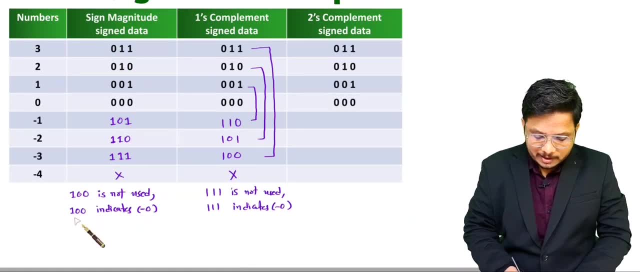 Like you see in 3 bit representation, we have wasted this number, that is, 1 0 0.. In 1's complement we have wasted 1 1 1, that is indicating minus 0. So here we are wasting 1 digit right. 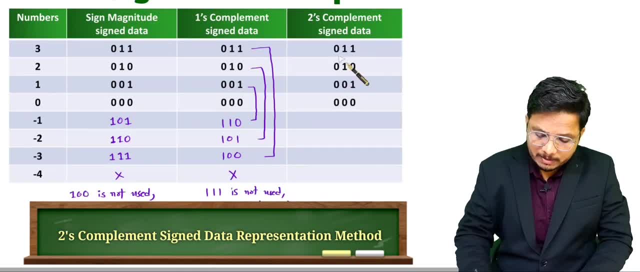 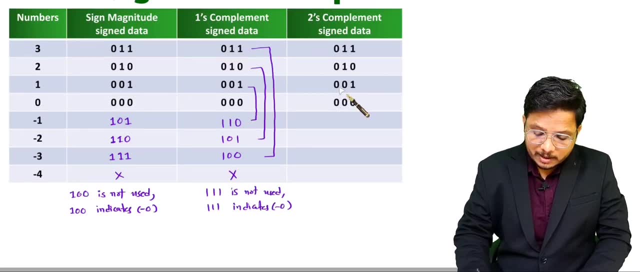 Now let us see how 2's complement is 0.. Yes, 2's complement method is there. So in 2's complement method, my dear students, to understand numbers you will have to take 2's complement right. So here you see, minus 1 that we need to have. 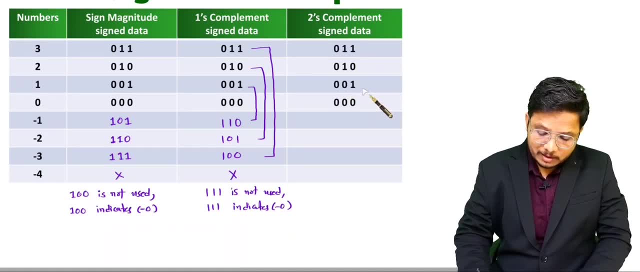 So to have that, you will have to take 2's compliment of plus 1.. So to have minus 1, we will be taking 2's complement of plus 1.. So here you will have to do what You will have to take. 2's complement means 1's complement plus 1.. 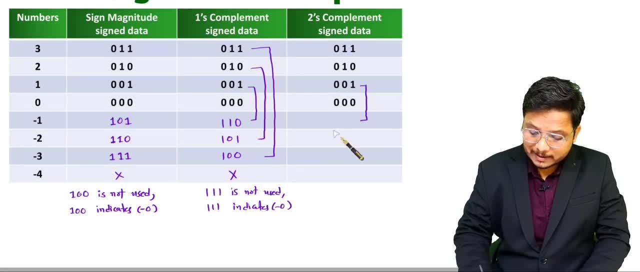 So 1's complement that we have already done, you see. So plus 1.. is 1, 1, 1, right: 1, 1, 0 plus 1, that is 1, 1, 1.. Then to have minus 2, you'll have to. 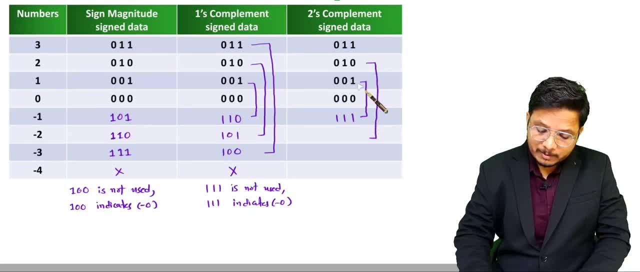 take 2's compliment of this right. So 2's compliment is what? 1's compliment plus 1.. So 1, 0, 1 plus 1,, that will be 1, 1, 0, right, And 2's compliment of minus 3,, that will be. 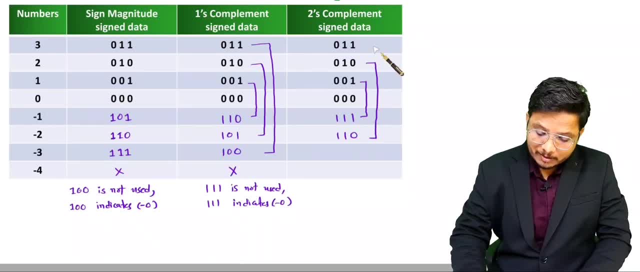 plus 3 and 2's compliment of plus 3, that will be minus 3.. So you'll have to take 2's complement of this. so that is what one's complement plus one, so that will be one zero one. now, my dear. 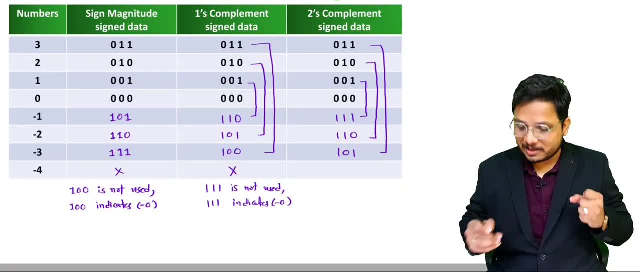 students, you might be having question, like what will happen with another digit. so here, my dear students, two's complement of four, that will be minus four, right, but if you observe here, we don't have four available over here as there is a limitation. but it is not like we are wasting. 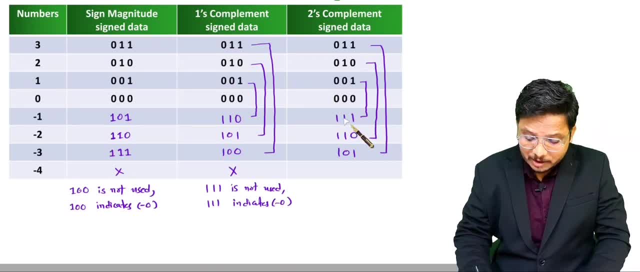 digit- over here you see how which digit- which we are not using till now. so if you observe, we have not used one zero zero right now. let me mention that over here: one zero zero that we have not used till now. now what will happen with one zero zero? if you take two's complement of this, then